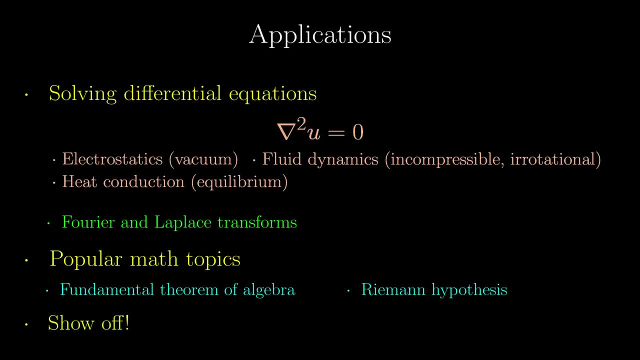 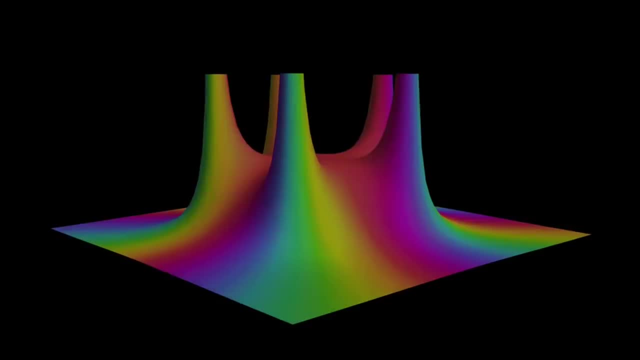 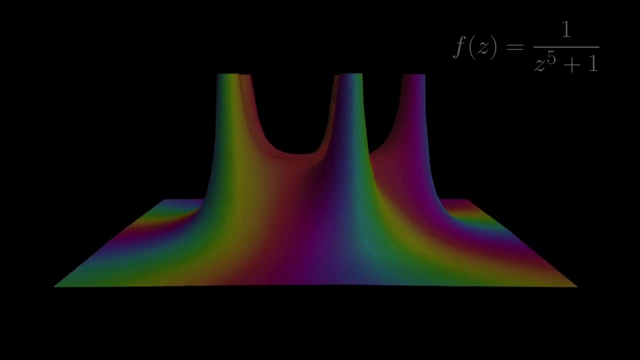 attractive enough. it allows you to show off. No, seriously, how would you evaluate this integral? Using partial fractions would be a nightmare, but if we consider its complex version, integrating on a complex plane, it becomes massively easier. And actually these are only applications that. 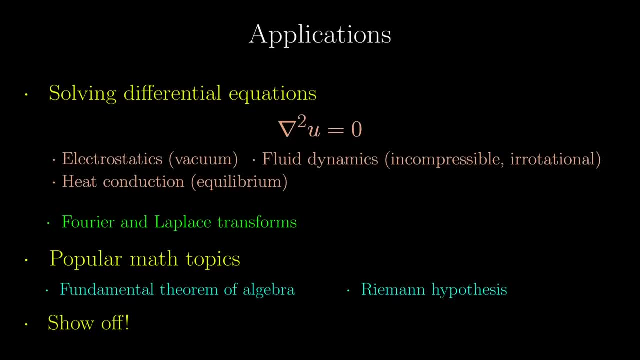 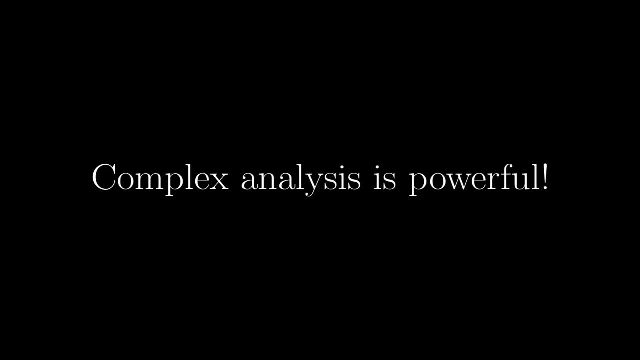 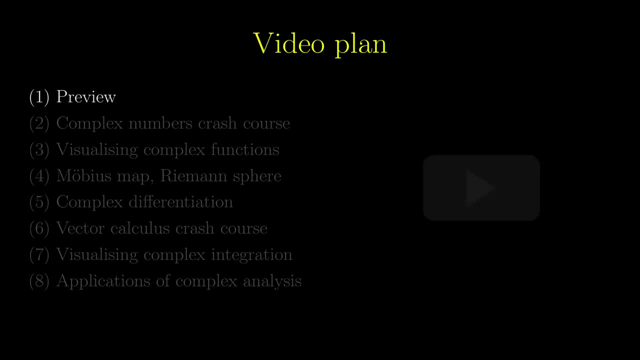 hopefully most of you would find interesting, but obviously there are more. All I am trying to say is that complex analysis is very powerful, And so I am going to make a video series about complex analysis, and this is my plan. The first one is this video: a preview of what's coming next. 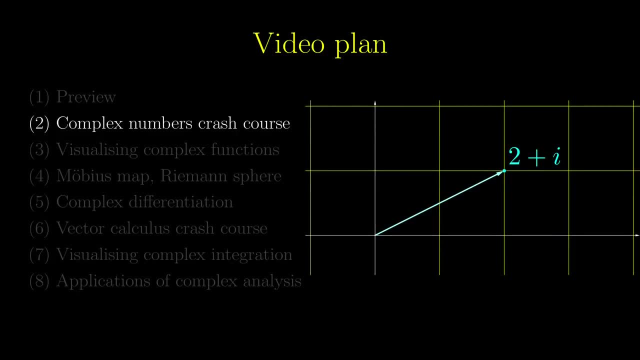 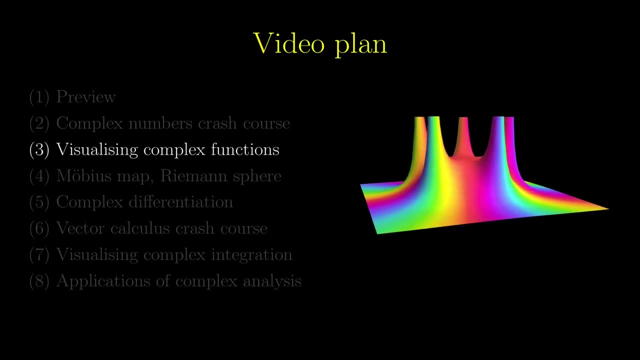 then a crash course on complex numbers so that we can all be on the same page, and then how to visualise complex functions and the messy stuff about complex functions. And then a particular kind of complex function: the Moebius map and the slick way of visualising it using the Riemann sphere. 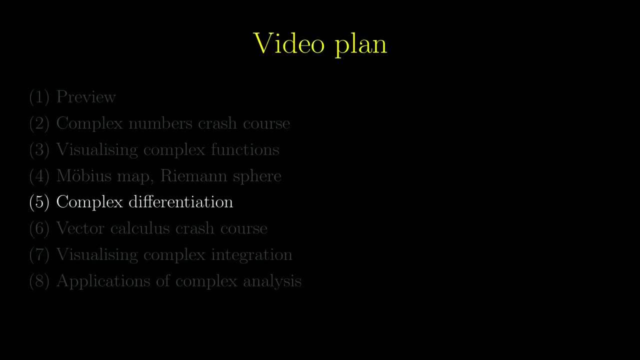 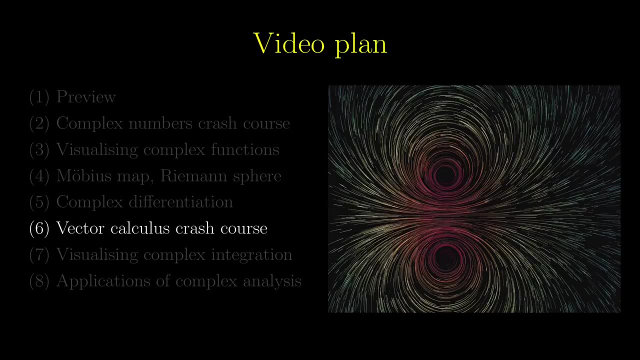 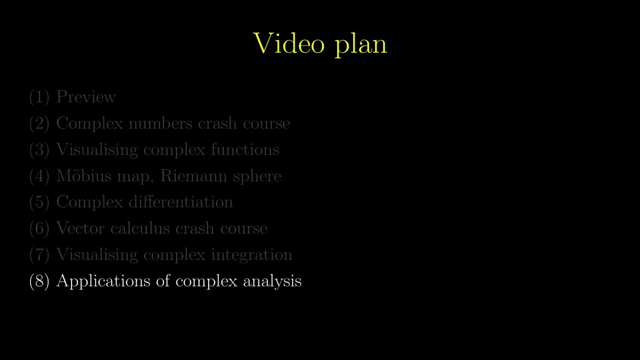 We can't not talk about complex differentiation, but it turns out that if we want to visualise integration we also have to know a bit of vector calculus first. But after all these we are going to see some of the applications mentioned, possibly in several videos. 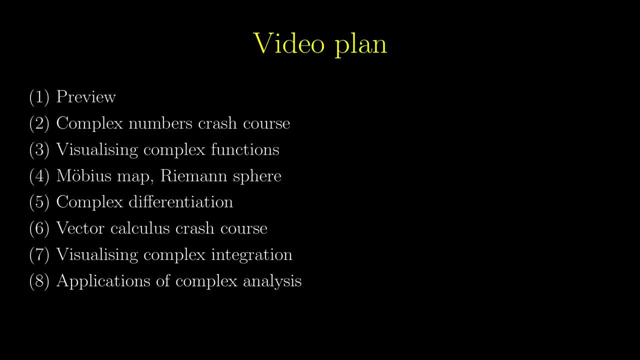 However, I want to emphasise that it isn't like this hasn't been seen anywhere on YouTube. Welch Labs made a series on complex numbers and functions. Moebius transformations were illustrated more than 10 years ago in this video. Zach Storr made a video on complex derivatives. 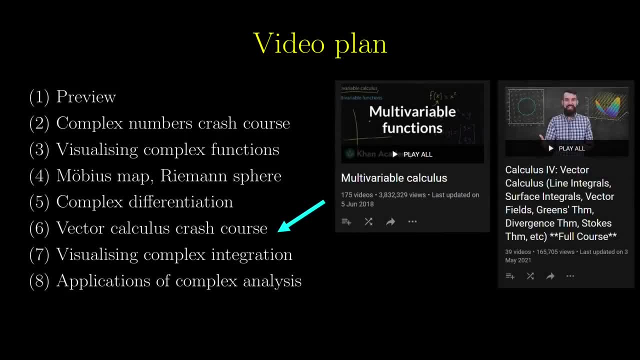 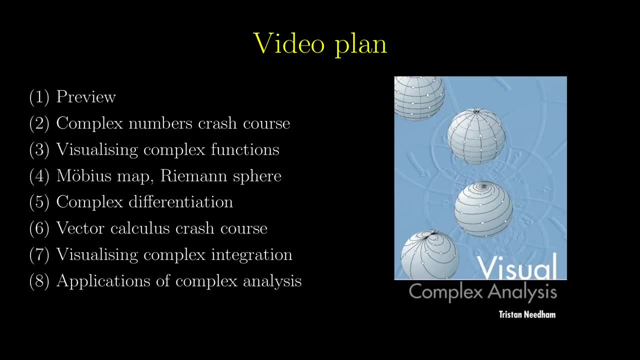 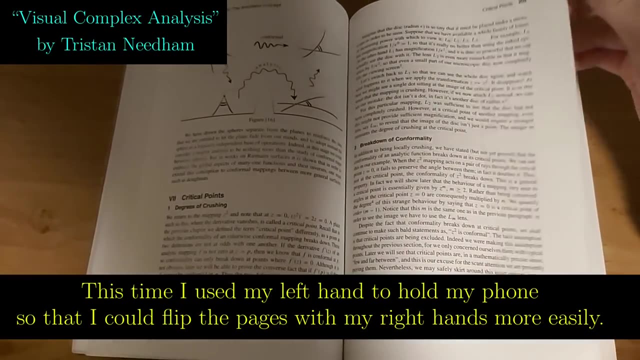 and so on. Loads of people have covered vector calculus before and actually this whole series will be very much from this amazing book called Visual Complex Analysis by Tristan Needham. So think of this series as a more convenient compilation and my take and animation on. 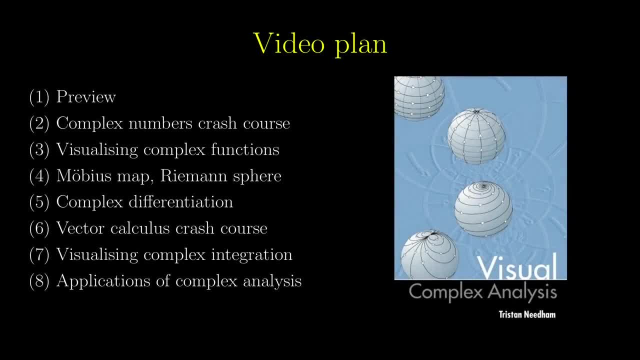 this subject. However, a little note that might be disappointing to the purists. This video focuses much more on visual insights and the rigor is not prioritised in the arguments. By all means make the arguments in the videos more rigorous, but in any case, I hope you. 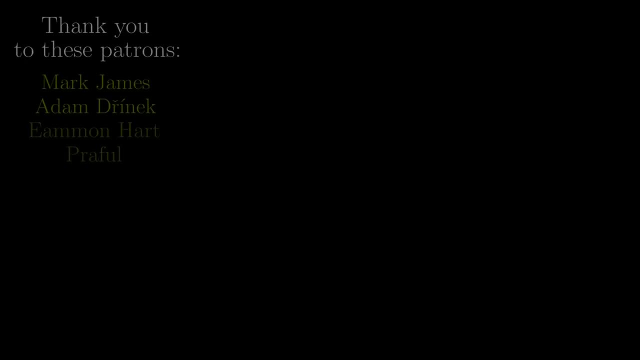 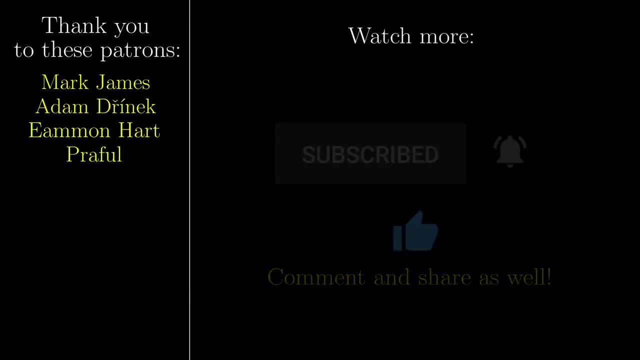 will enjoy the series ahead Thanks to these Patrons and, as always, like and subscribe with notifications on comment and share the video as well. See you next time. Subtitles by the Amaraorg community.